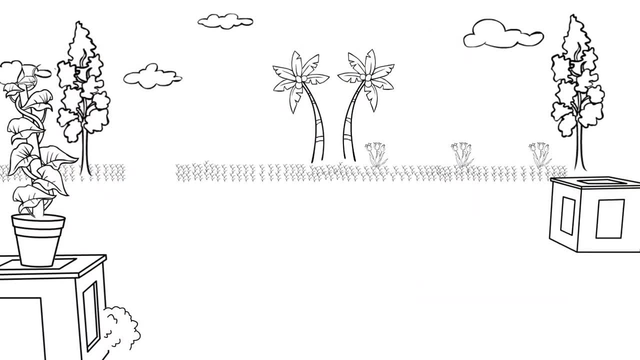 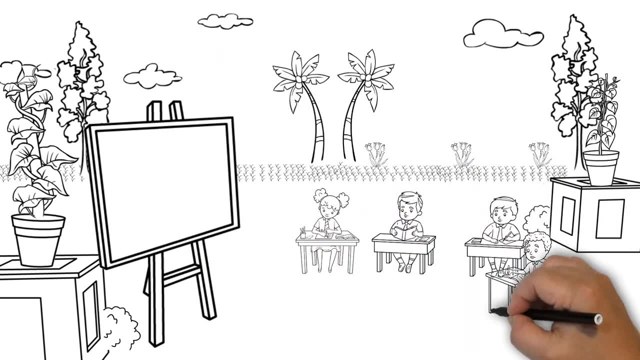 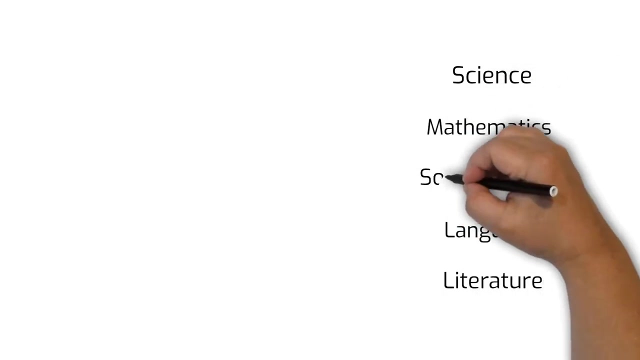 Why philosophy for children? After all, children are burdened with so many subjects. You have to read subjects like mathematics, science, social science, literature, language, and where is there space for learning another subject? But philosophy is not another subject. Philosophy, rightly, can be. 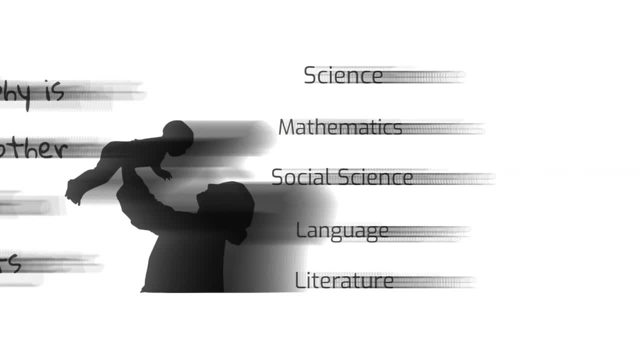 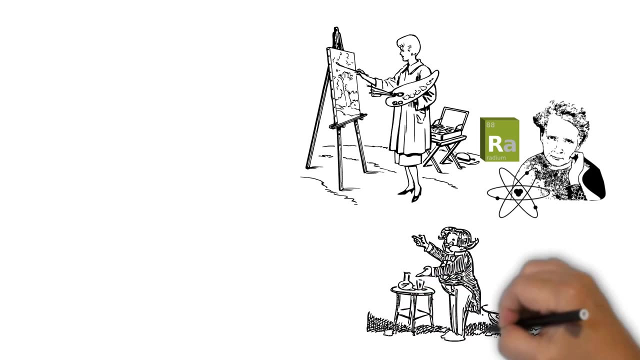 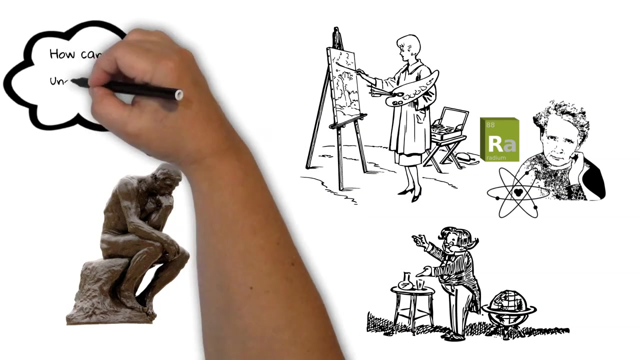 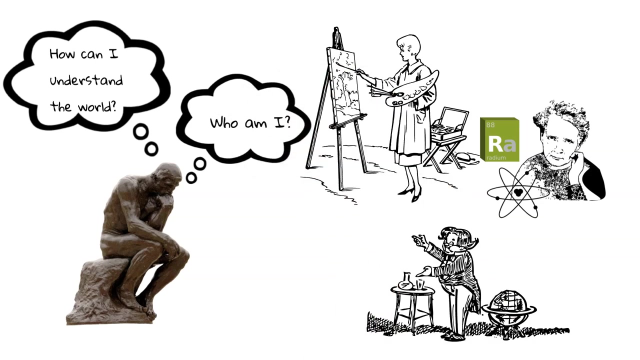 called as a mother of all subjects. Much before subjects like science and maths and arts and social sciences began, what was present was philosophy as a discipline, Philosophy as an idea, Philosophy as something by which people understood the world and understood themselves. All subjects, in a sense, are children of mother, a mother called philosophy. So today we may not. 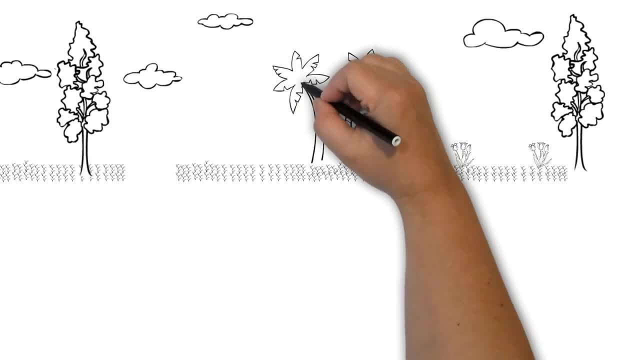 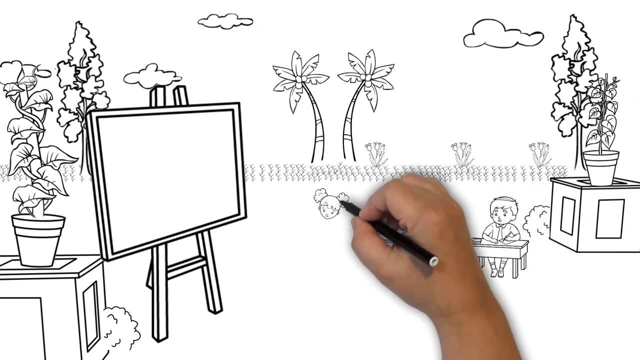 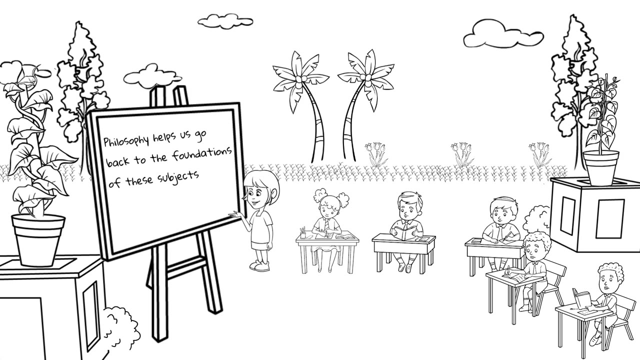 teach philosophy in schools because we are interested in just looking at all the other subjects which have come from it. But we are at a time in our world where it is necessary to go back and think about the beginning of these subjects, Think about the foundations of these subjects. 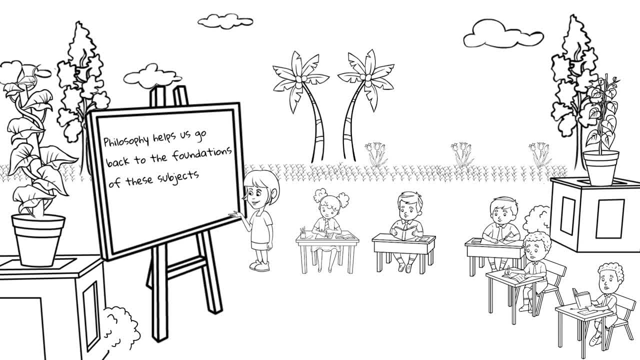 To do that you have to go back to philosophy. There's another reason why philosophy is so important for children: Because the basic, fundamental idea of philosophy, the way of thinking philosophically, is always present in children. It is children who ask very inconvenient questions, Children who can see the world. 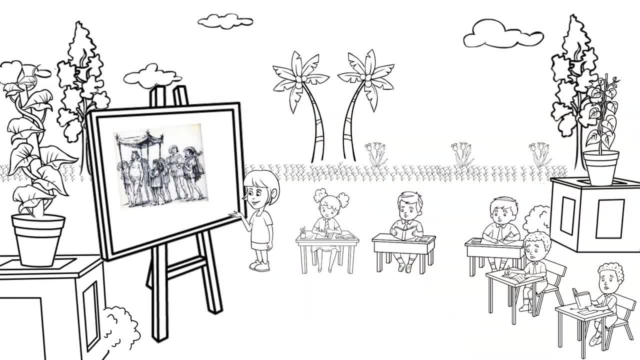 differently from that of the adults, Children, who can make you say, when the emperor has no clothes, without hesitation. And that way of thinking and looking at the world is where philosophy comes from. And that way of thinking and looking at the world is where philosophy comes from. 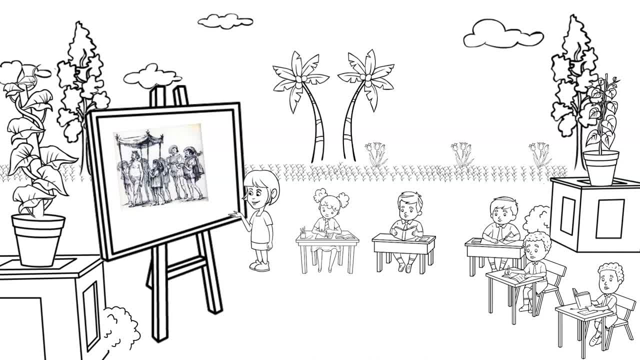 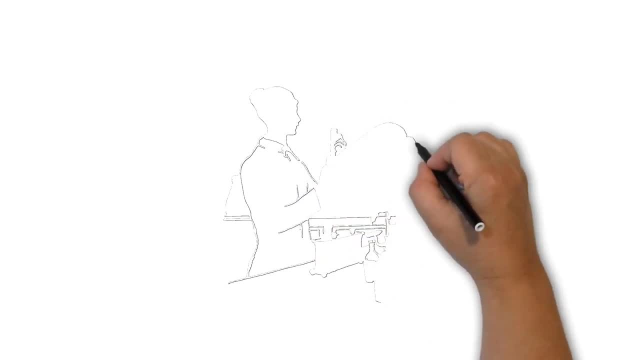 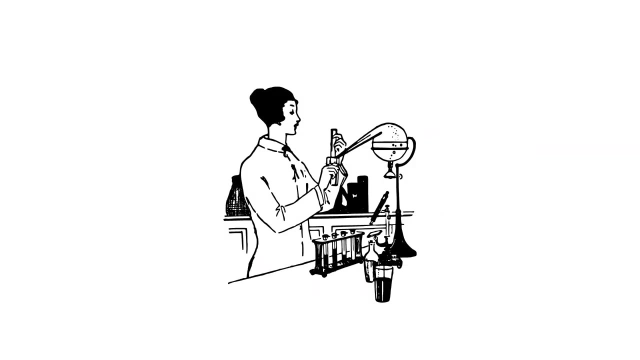 And why is this way of looking at the world important for us today? It is important because through philosophy, we can actually understand these various subjects. So what subjects do is tell you something, give you some knowledge and truth about certain aspects of the world, And what science can do is to give you some information about the nature of our world. 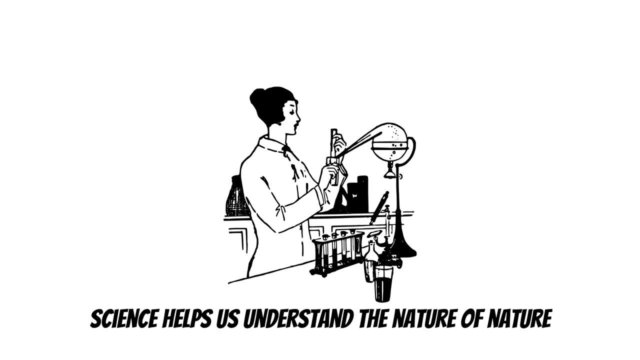 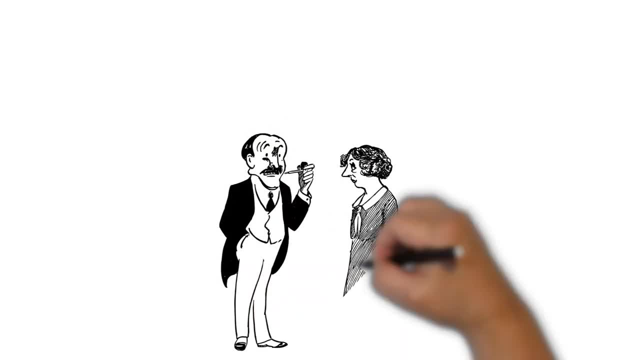 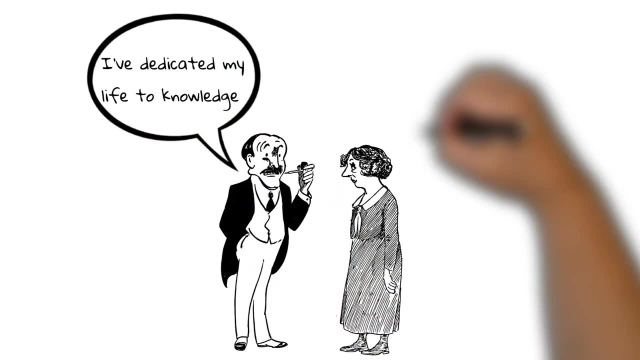 if you like, What the nature of nature itself is. But to understand what these subjects are, to have a better understanding of why subjects are different from each other, what is special to each of them, we need to go back to philosophy. And that is the strength of philosophy, Because it gives us far better understanding, It makes 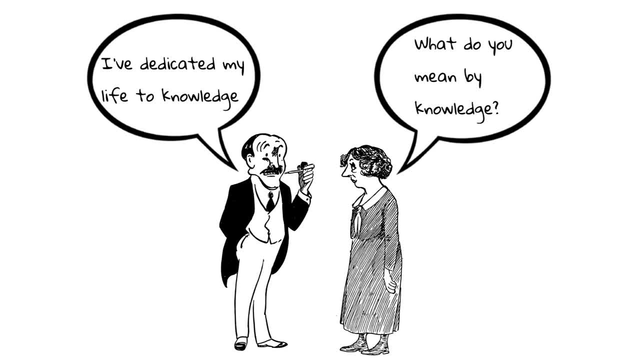 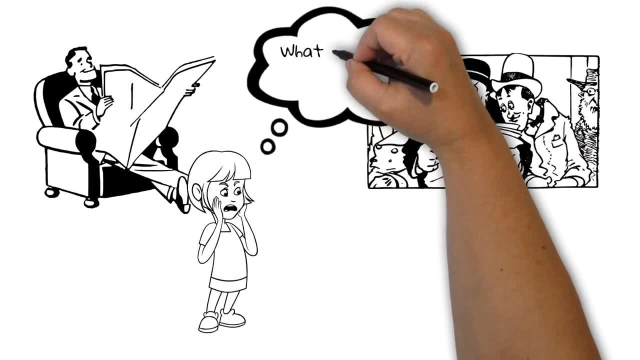 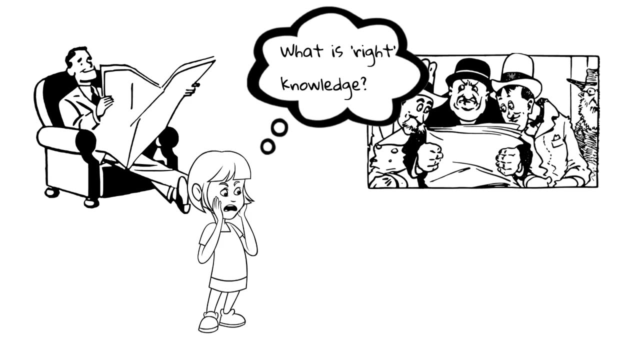 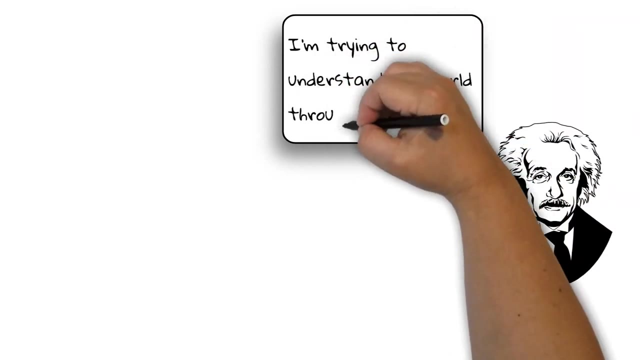 us aware not just of what the knowledge is, but how we produce that knowledge. And that is a very important skill which is necessary in a world which is now completely overflowing with too many specializations and too much knowledge from everywhere. So look at this example of science. If science is about understanding the world, then one could say: 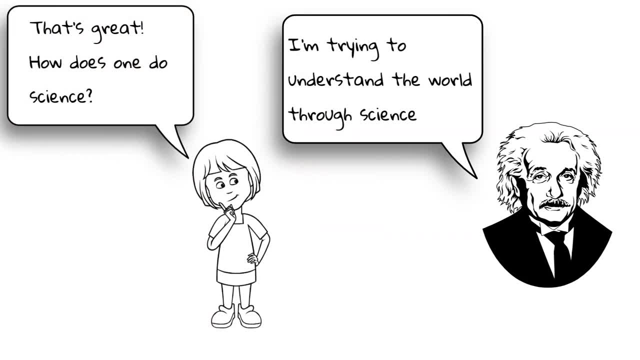 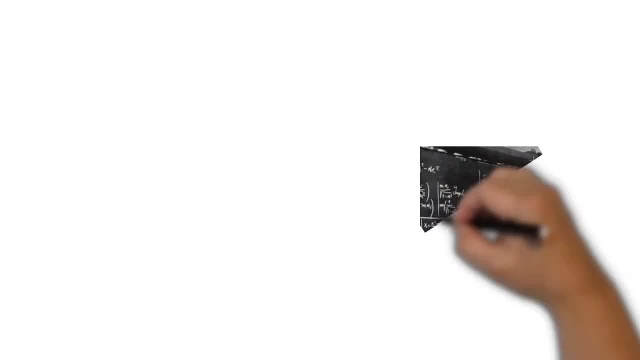 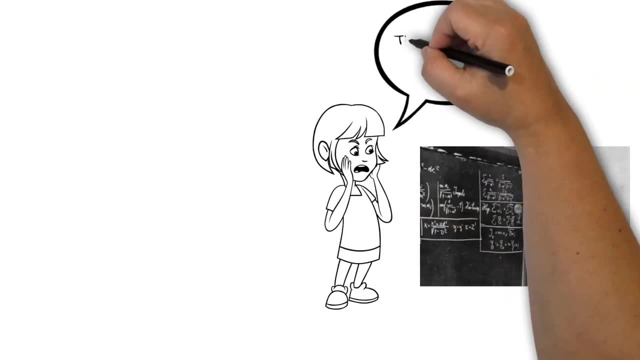 philosophy will help us understand science itself, What science is doing, Why science does what it does. For example, why does science use mathematics? Why is mathematics so important for science? Now you might think in your own classroom. when you do science, you do your class in a very different. 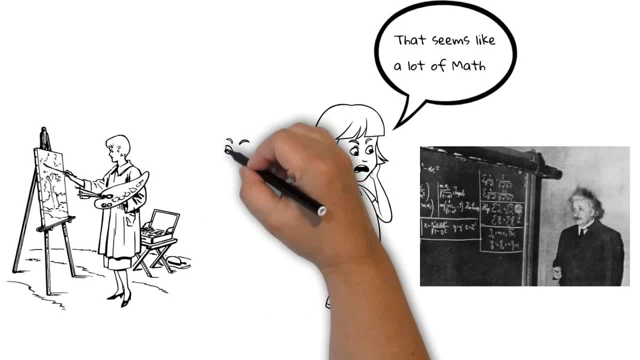 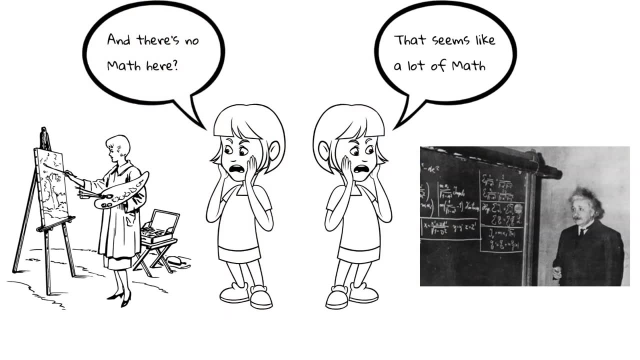 manner. You do calculations, you solve problems and so on, But when you are in your music class or English class, you might do it very differently. So you have to ask yourself: why are these subjects so different? What is special that these subjects do these? 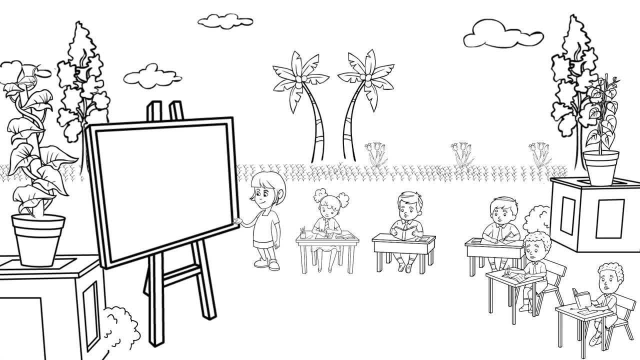 things in a very different manner. So philosophy is not interested in solving problems or solving equations. It is trying to understand why science does what it does And how is it that if you do those actions, you are able to produce knowledge about the world? You know there are many terms. 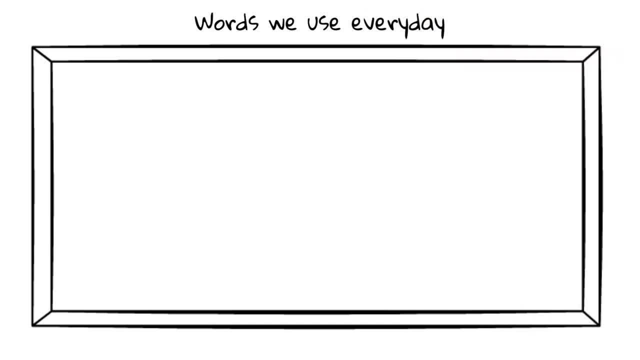 we use in our daily lives. You use in your own day to day talk with your friends and in your class and with your family. You use in your own day to day talk with your friends and in your class and with your family. I'm sure all of you use terms like truth and you will say: don't say lies, be truthful. 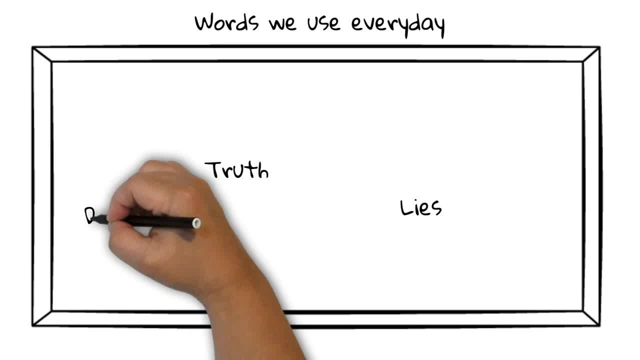 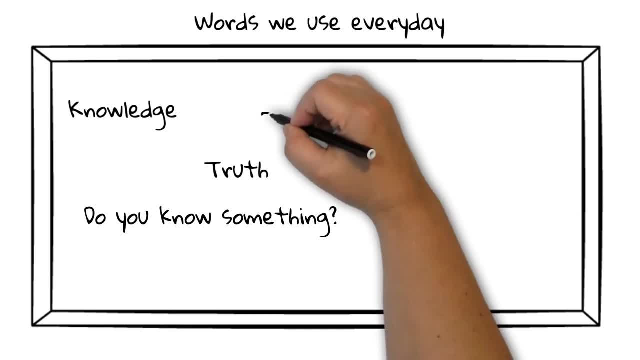 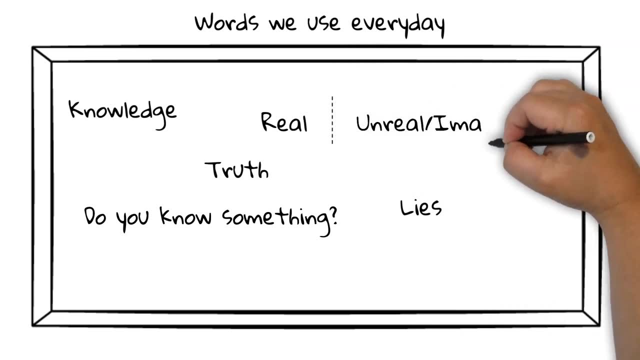 I'm sure you use terms like: do you know something? Terms like knowledge are very commonly used by us. Terms like real are also very much used by you, because something seems unreal, something seems imaginary to you, And children, I know, talk about imagination all the time. They are very fascinated. 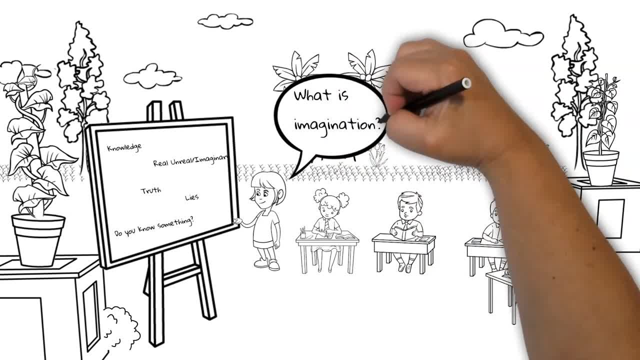 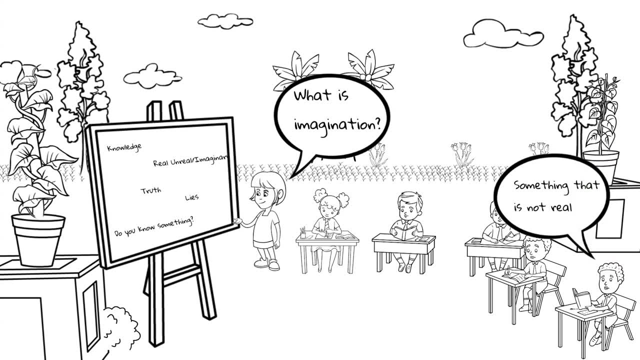 by imagination. they will never forget it. So you know- I'm sure you are writing it down- why I am saying so: imagination. But if you really ask them, what is this thing called imagination? Many times they say, well, imagination is not something that is real. So you have an idea you're working with. 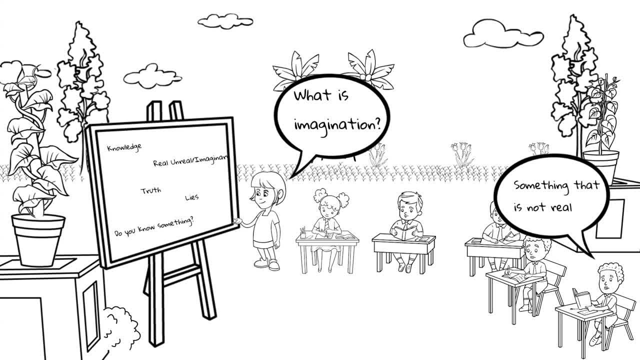 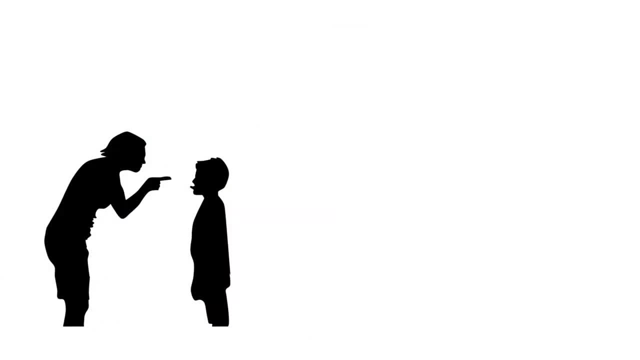 these thoughts about imagination, reality, knowledge, truth. And then you're also confronted by so many things adults tell you, both in the family and in your schools. They'll tell you to behave in a good manner, be good, And then you wonder and say, what is it to be good? 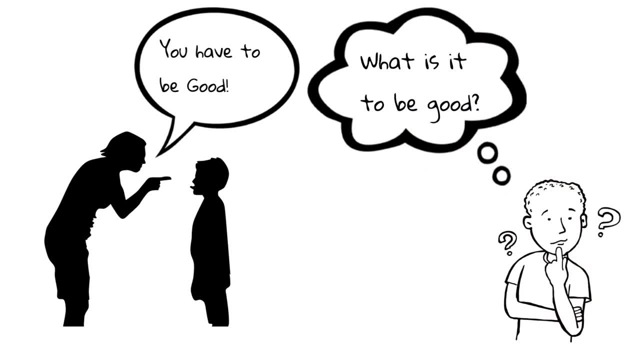 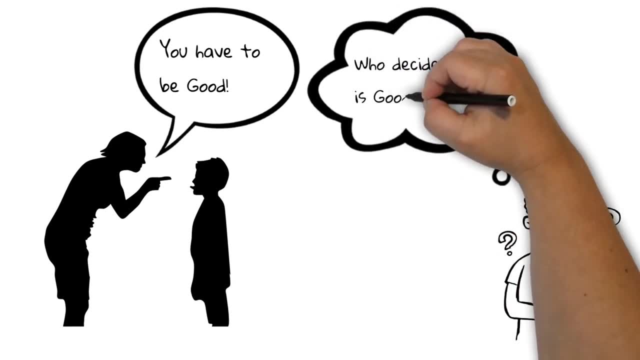 And why are adults just bothering me so much about being good, telling you all the time: be good. So what is it to be good? How do you know when you're to be good and not to be good? And who defines that? Is it only adults, who know what is it to be good? So this is a question. 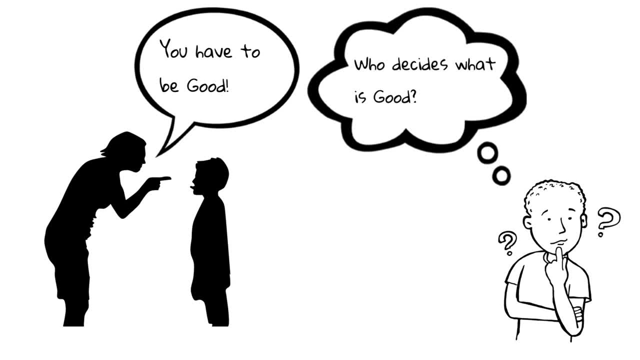 which is also very important philosophical question. You're already thinking about it. You may not be thinking about it Saying, oh, I'm doing philosophy. You know you don't have to do it like that. It's not like doing science, like when you decide to solve a problem. You're thinking philosophically. when you're. 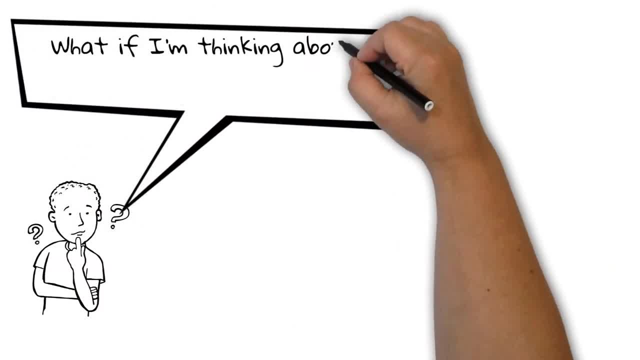 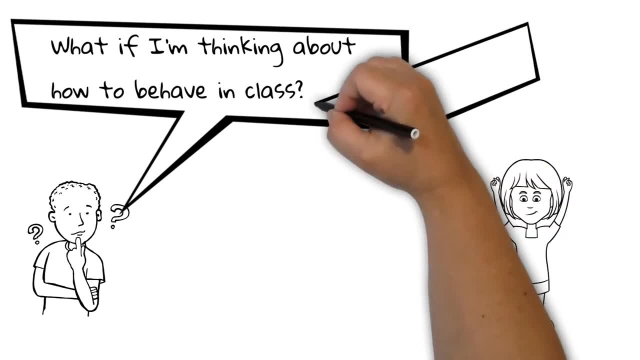 thinking about these questions, when you're thinking about what you should do, how you should behave. Suppose you see something in your class and you feel: oh, how should I behave in this circumstance? You're already asking, in a sense, a philosophical question. When you learn language, 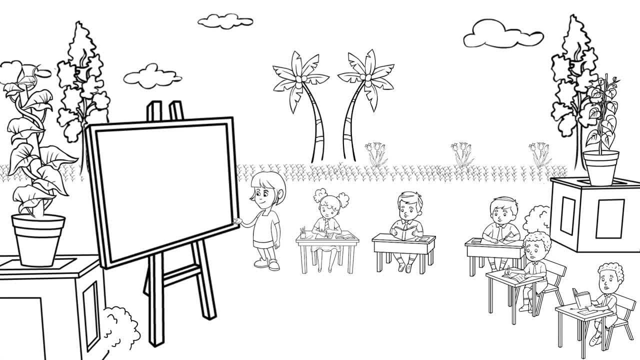 you learn new words And you say, when you read a classroom book, a text in your class and you say: oh, I don't understand this lesson, Then you're asking yourself: why am I not understanding that lesson? Is it because of the words which are used in it, Or is it because there is something called? 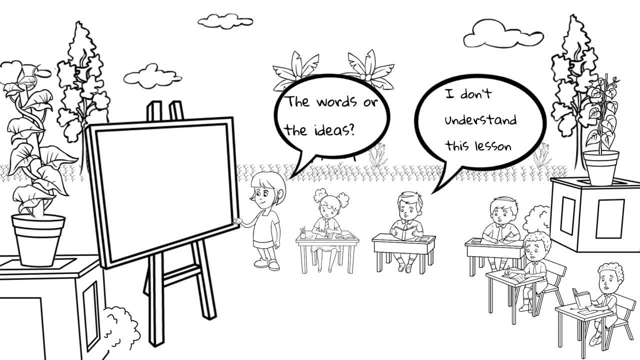 an idea which is hidden inside this language. So what is language itself? How do we understand? We use language all the time, but how do we understand The nature of language As children? there is something else you do all the time. 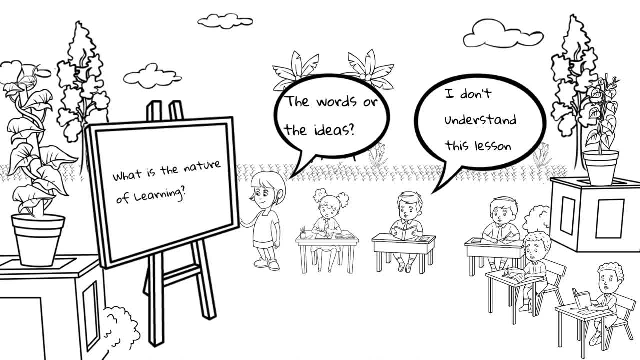 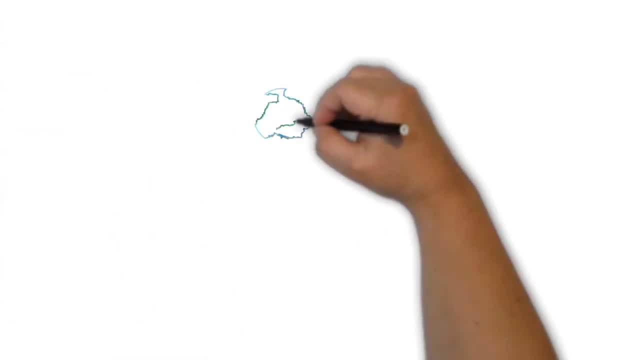 and that is this act of learning. So what is it to learn then? You know, everybody tells you learn this, read a book. Is just reading a book learning? Or have you ever wondered: could learning be something slightly different? Like you might have read, let's say, the earth? 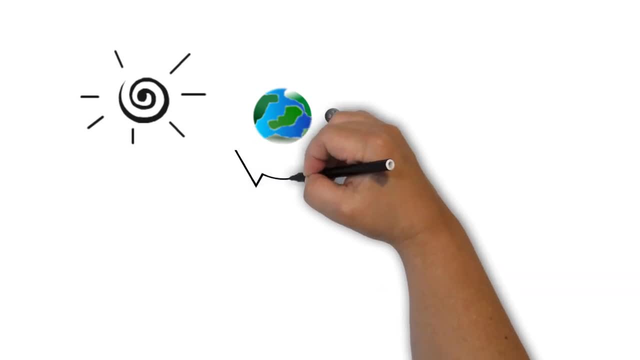 goes around the sun. It revolves around the sun. Everybody seems to be sure that the earth revolves around the sun, You know, but I am not so sure, actually, because I don't know how to understand how the earth revolves around the sun. Is there some hidden force? Is there a hidden, some hidden invisible? 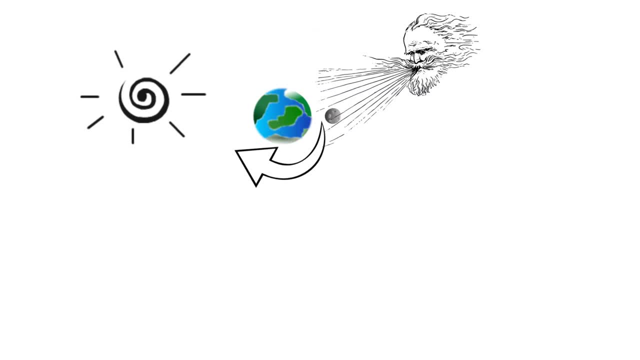 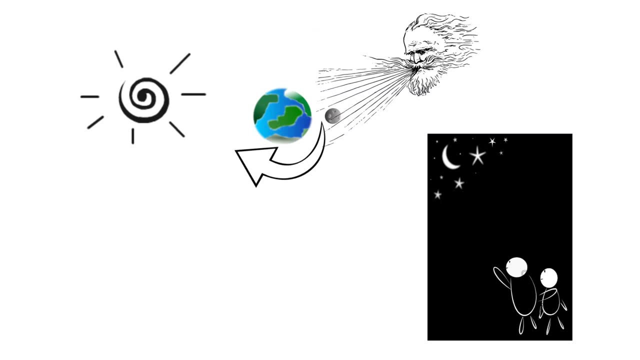 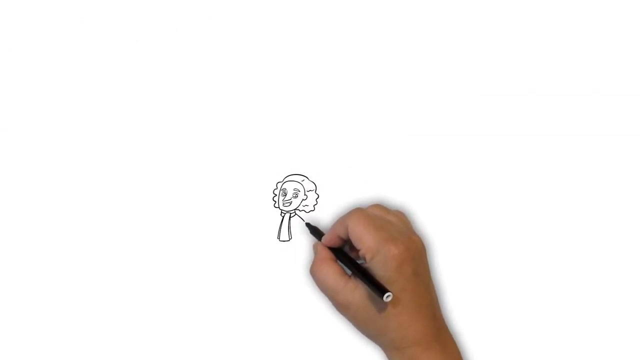 hand. Now, this is not just about telling a story. This is how the first beginnings of physics happens, when Newton is asking this question. After all, the sun and the earth are not the same, They are not attached to each other, And Newton is thinking of an example like a stone at the end of 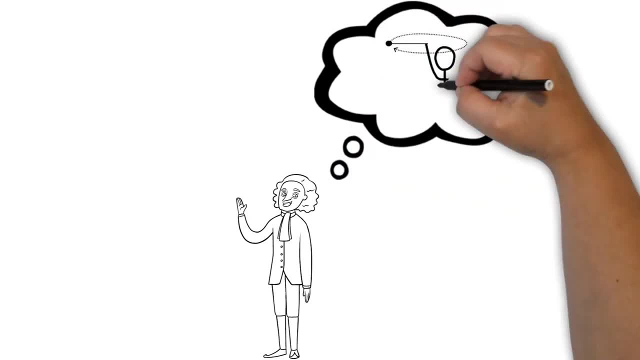 a string. So if you take a stone at the end of a string and you keep whirling it as you do when we play games, you know you can whirl it around very fast. So maybe the earth is like the stone attached to the end of the string and the earth is going around and around the sun And Newton. 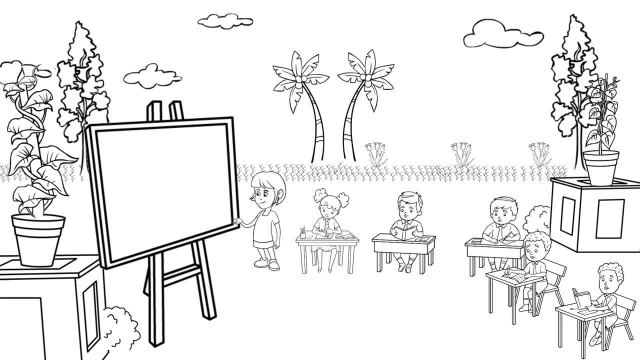 actually thinks of this image. So what is it to learn? So it is learning just to say the earth is going around the sun, or is learning something more? Is it about knowing why the earth goes around the sun? It's not just to know the answer. Learning is not about knowing the correct. 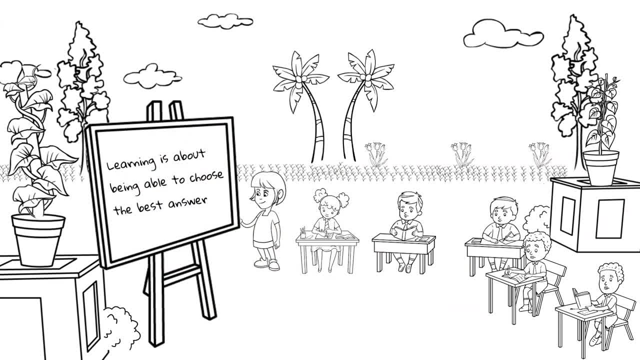 answer. That's not learning. Learning is when you can think of different answers and you are able to choose what seems to be the best answer among all these other answers. So learning is actually something which is very philosophical in nature. So when you are sitting in classroom and learning all these facts and say learning like 2 plus 2 is, 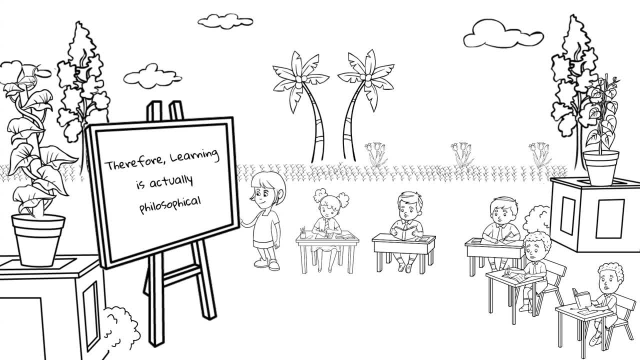 4,. the moment you start asking: what am I actually learning? Why is 2 and 2?? If I add them, why do they give something called 4?? Can I apply this knowledge to the world? Can I use this knowledge? 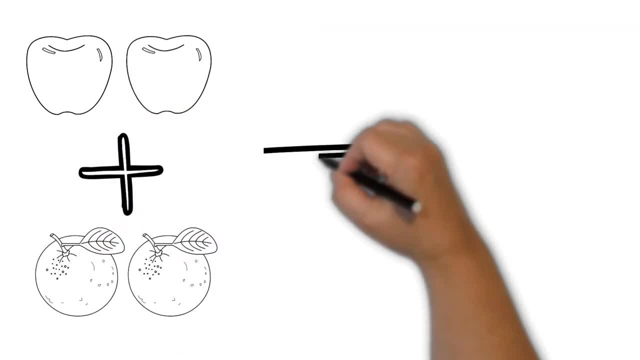 to say, well, if I take two apples and two oranges, then I will have 4.. And that's not a simple point, because if I add two apples and two apples I can get 4 apples. But if I add two apples and two, 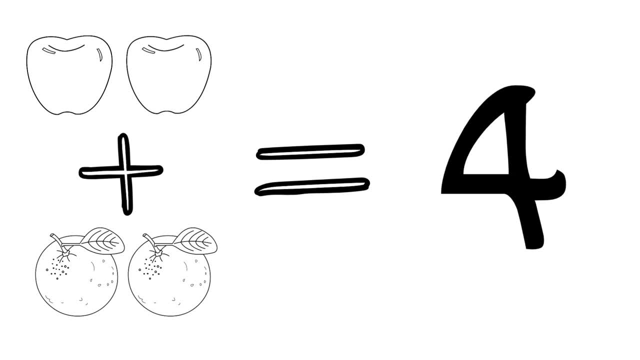 oranges, I get something called 4.. But you can't say it's 4 apples or 4 oranges. You think about this very subtle jump. What you'll have to say is, if I add two apples and two oranges, I'll get 4. 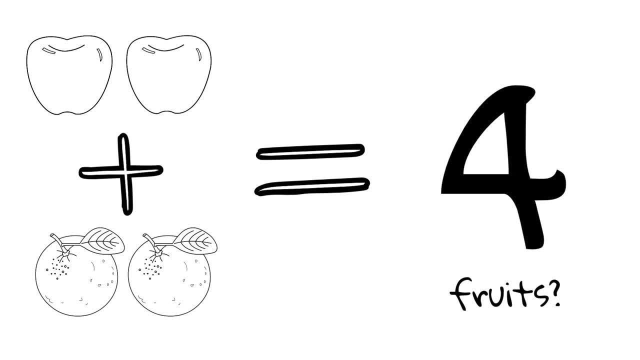 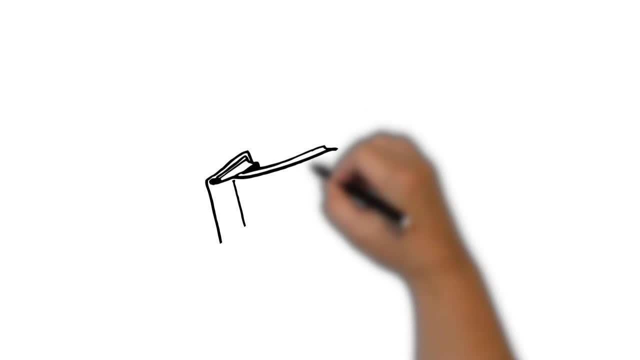 fruits, And if you don't have this concept called fruit, then 2 plus 2 is really not equal to 4 in this case. So what I would say, as at the level of thinking about philosophy for children, is that all these are ways by which we 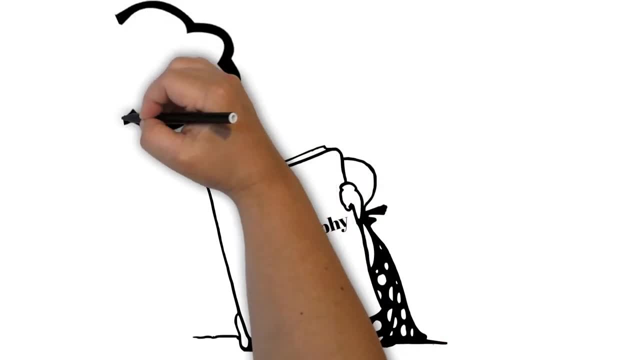 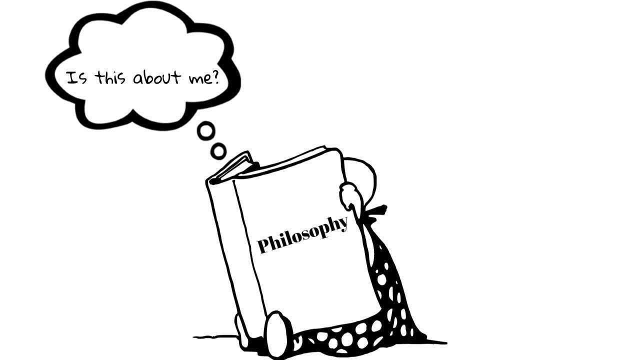 introduce a child, somebody who is in the class, who's learning new things, about becoming aware of themselves when they learn. So there's a lot of philosophy which is about this awareness and self-awareness, becoming more careful about what you believe, how you believe something. 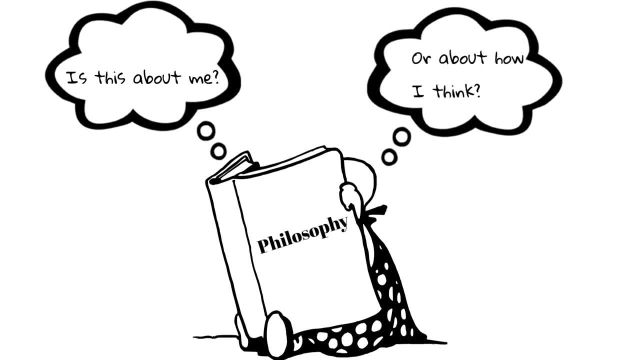 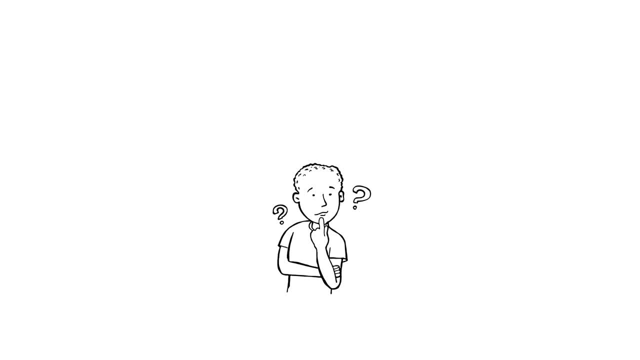 what you accept, how you accept a particular idea And so on. And a very important aspect of this, this task of philosophy, is not just to understand something about the world, which is very important, which is what science does, something about society, which is what social science does, you know, producing new ideas in language and 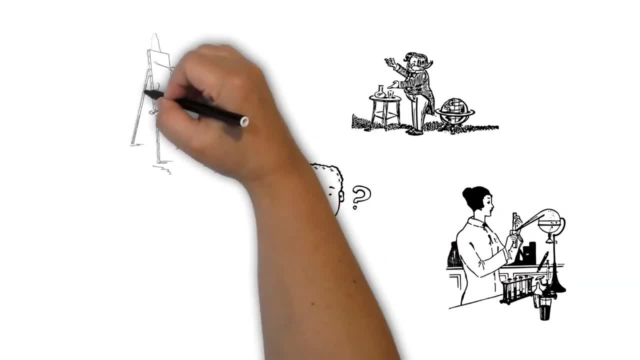 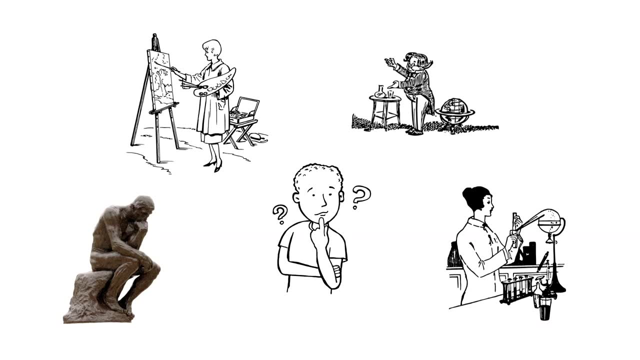 mathematics and so on. All these are very important, And also, for example, art producing new art. But a central core of philosophy is also to understand the nature of who we are. After all, it's humans who are producing this knowledge about the world. 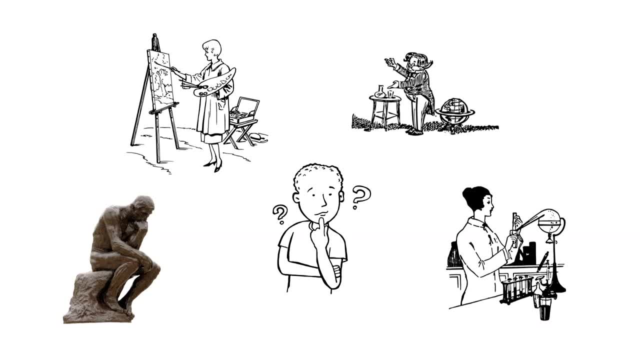 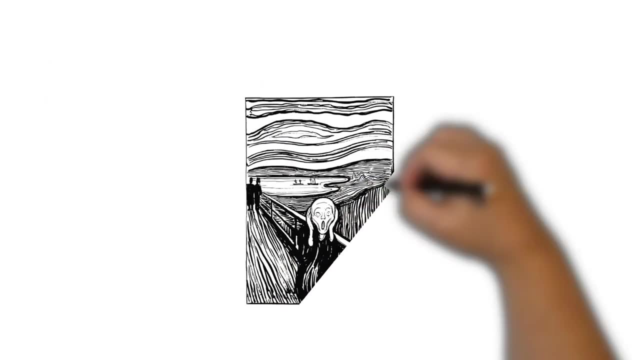 It's humans who are telling you that the earth is going around the sun. It's humans who are telling you that 2 plus 2 equal to 4.. So who are these humans? Why do we produce this kind of knowledge? How is it possible that we are able to do it? And I'm sure every child in us is asked this question. 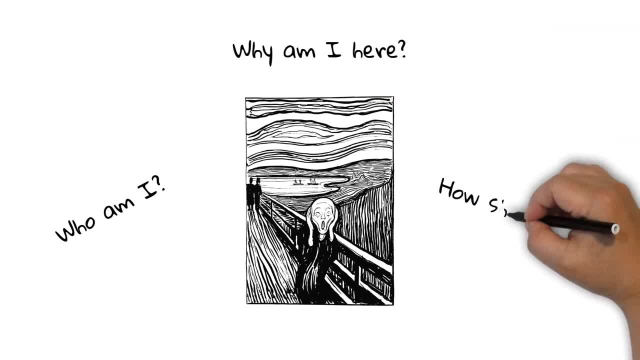 at some time or the other. Who are we? What are we doing here? What is our role? What should I do, How should I act, How should I behave, How should I think? All these are very fundamental questions of who we are, And that question is central to 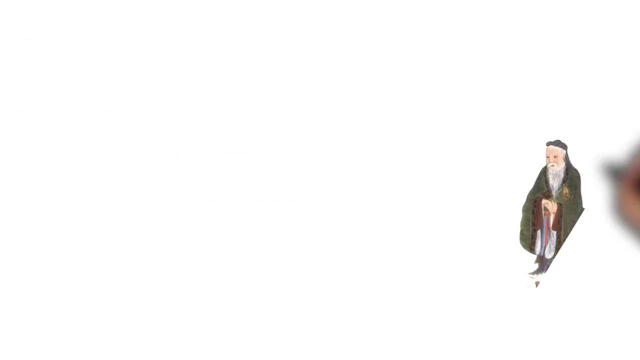 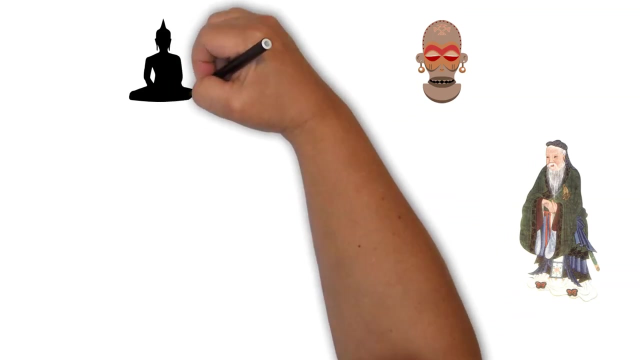 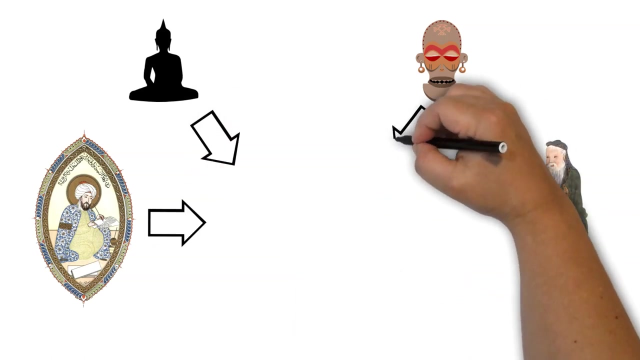 philosophy, Every philosophical tradition in every civilization brings the human in the center of the world, And that's a very important aspect you have to remember. That is, philosophy as a way of thinking and of knowing includes not just the world we live in, the universe we are part of. 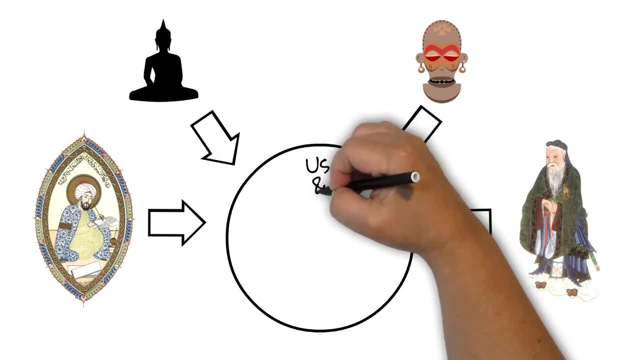 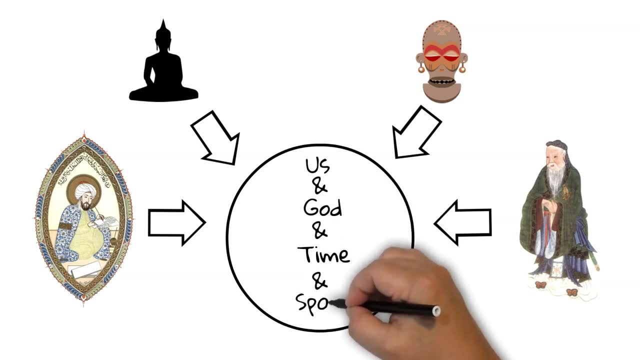 it includes ourselves. it can include things which we cannot see. They can talk about things like God. they can talk about things like time and space. All of these become very important And we have to to remember that philosophy is not just a byproduct of one culture, Every culture. 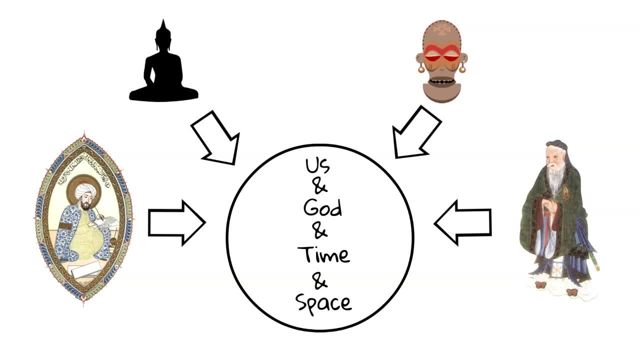 every community produces its philosophy, this way of thinking about themselves and about the world. They may be different, but they're all doing this job. So, although we hear a lot about Greek philosophy and Western philosophy, which is very important now for modern disciplines- 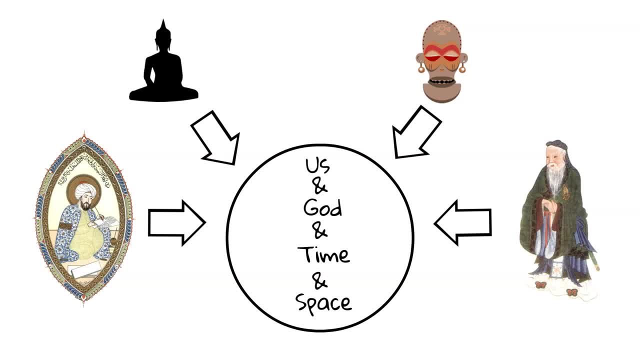 nevertheless, it is the case that, historically, that the most profound philosophy begins from Asia and Africa And there are many different ways, many different new ideas of philosophy which come from all these different civilizations. Very rich work is done, for example, in the many 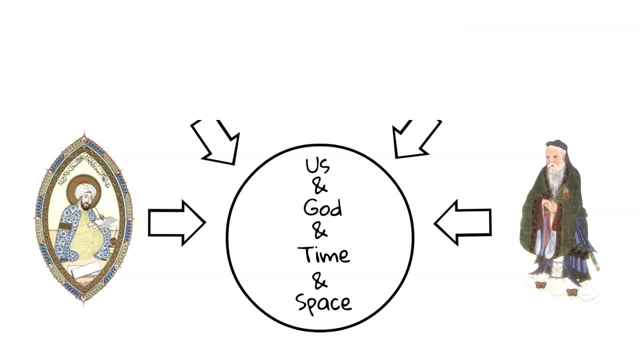 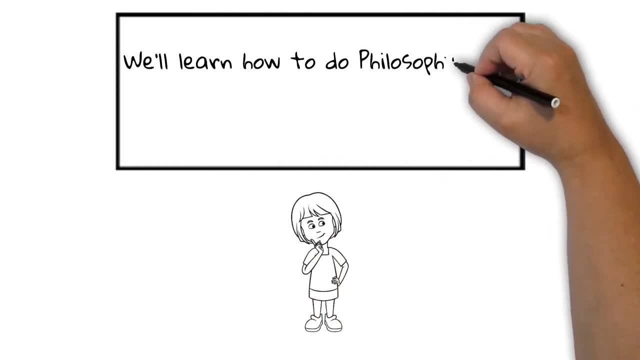 different Indian philosophical schools And, as we go along in these lessons, we will look at examples of different Indian philosophical schools And, as we go along in these lessons, we will look at examples from philosophy across the world to try and understand what philosophy does. 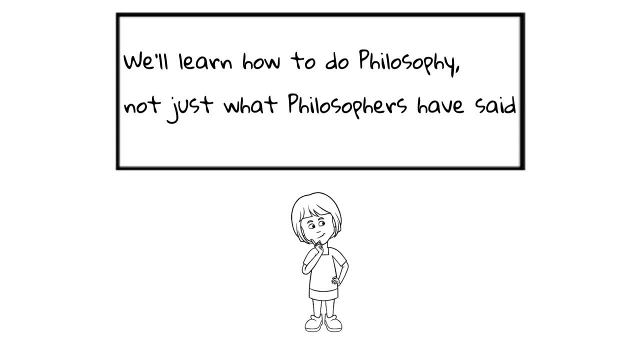 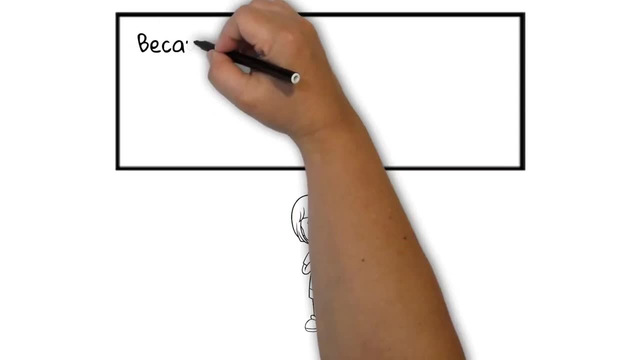 rather than reduce philosophy to some content of what philosophers said. Our interest here is not that. Our interest here is to ask: why do philosophers ask these questions? Why are they even thinking like this? What makes them ask these questions? And, as you can already see in, 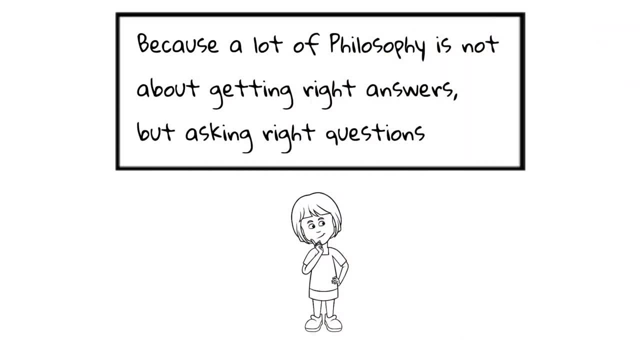 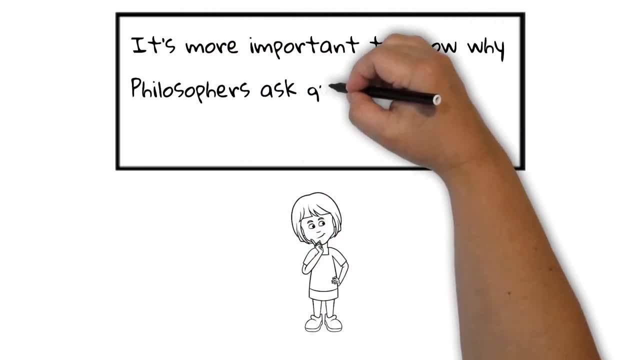 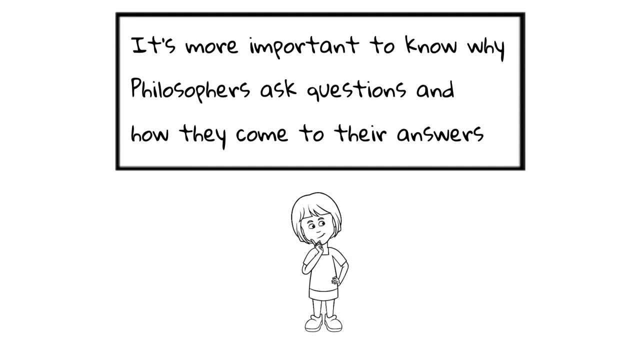 this short introduction. philosophy is a lot to do with asking questions. Thus, we should remember that when we read philosophy or when we think about philosophy, it is not as important to hold on to what one philosopher said or what somebody else said. It's more important that you understand why are they asking those questions? first of all, 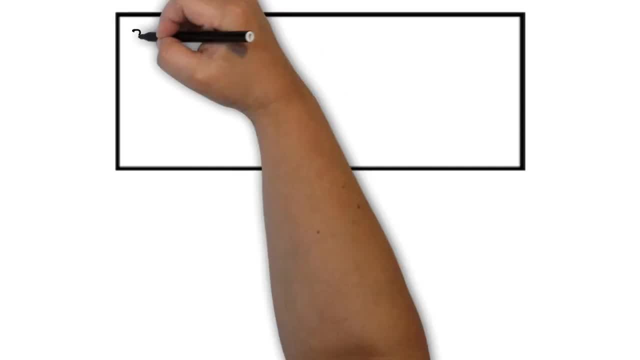 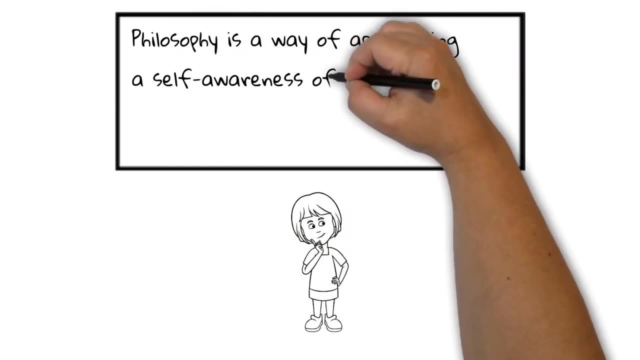 and how do they come to those answers? So, in conclusion, we could say that philosophy is a particular way of approaching a self-discipline, And that's why we should remember that when we read philosophy, we should know what it means and what thepless is, what philosophy is and Candidate.